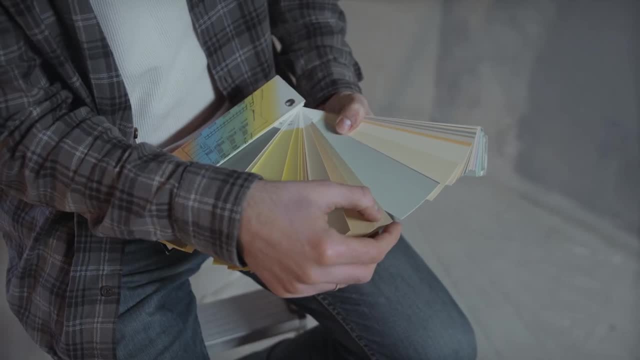 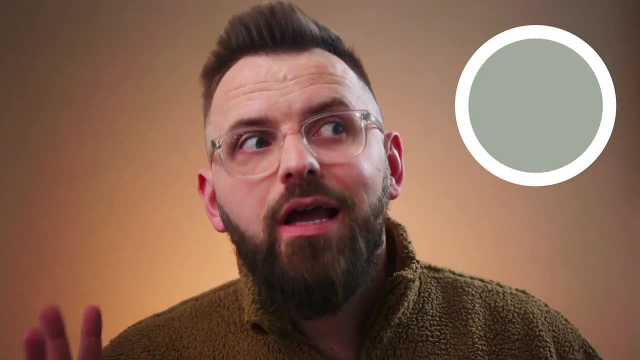 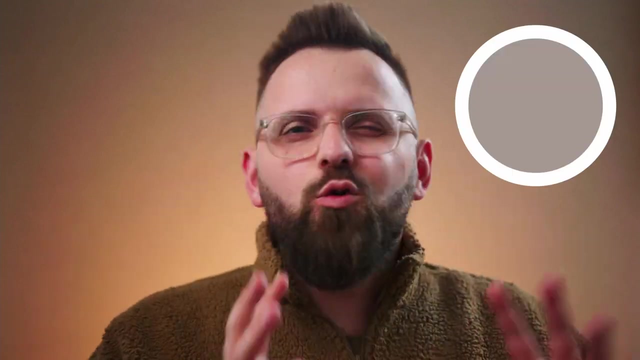 look like, But if you know anything about paint colors, gray can mean a ton of different things. You can have cooler gray, warmer grays, greeny grays, bluey grays. I even tried to make up subcategories like grouge, just to make things a bit easier. for myself, Grouge is a bit of a rougie gray or a red gray. 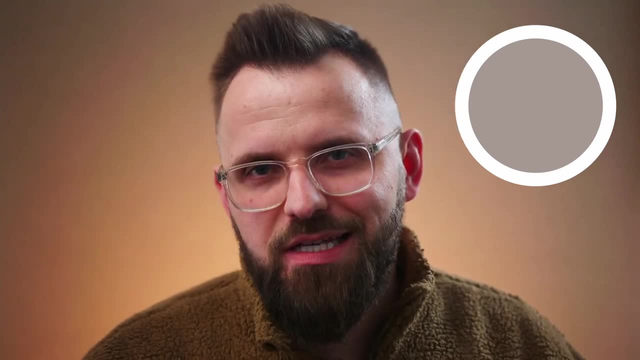 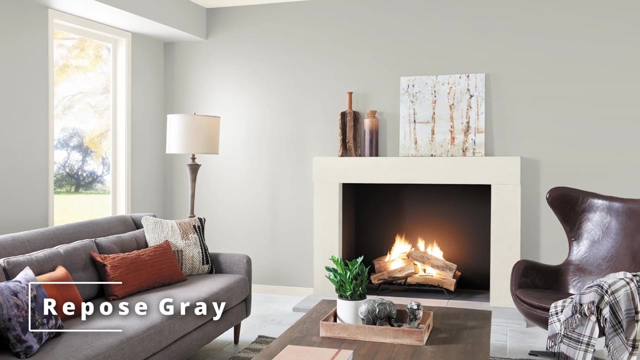 We did a video on it which I can leave in the cards up top if you're curious. So as for similarities, Repose Gray and Agreeable Gray do fit under the very broad umbrella that is gray. Another pretty clear similarity they have is how dark they are, or how light they are. 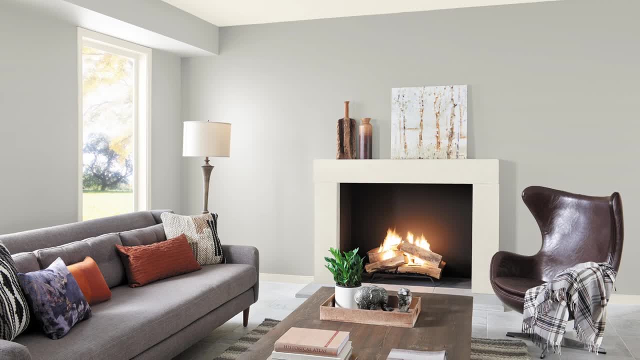 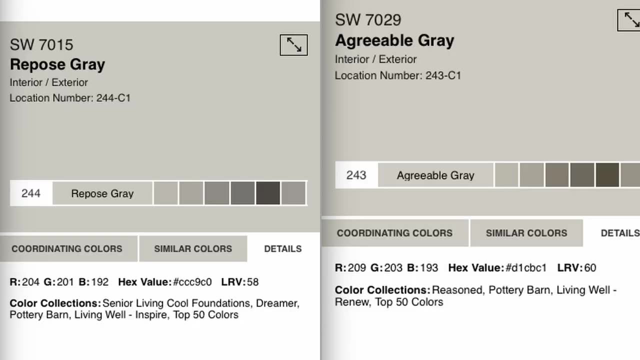 depending on how you put it. What's great about paint colors is you can actually find a very specific number on any paint company's website. So in this case, you go on the Sherwin-Williams website, you click on the details tab and you'll see something. 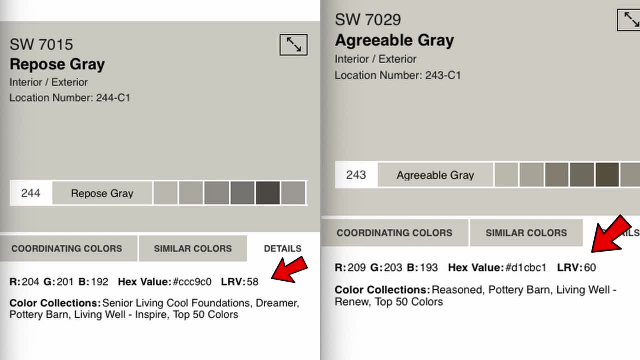 called the LRV, which stands for light reflectance value. You can do this with any color on the site. The light reflectance value is just a number between zero to 100, reflecting a percentage of how much light a certain color reflects, That is. 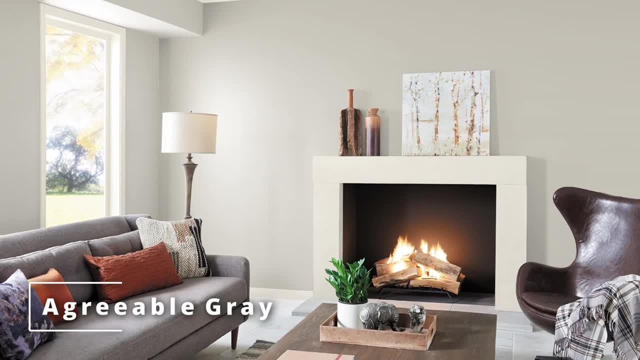 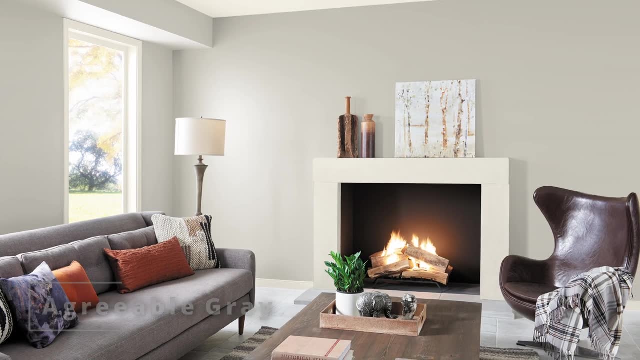 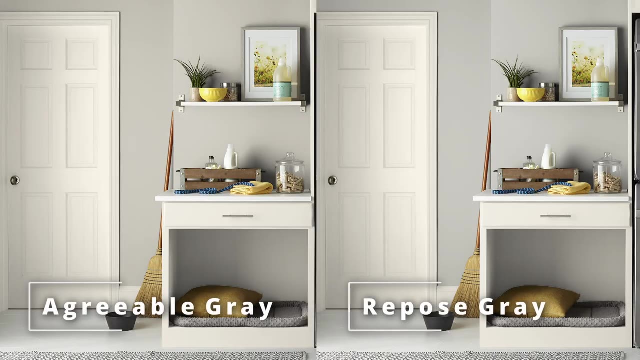 visible light, And why this information is useful is because a color that reflects more light will appear lighter to you. So the purest of pure whites might be close or approaching 100, and the deepest blackest of blacks will be closer to zero. Agreeable gray and repose gray hover around the 60 mark. 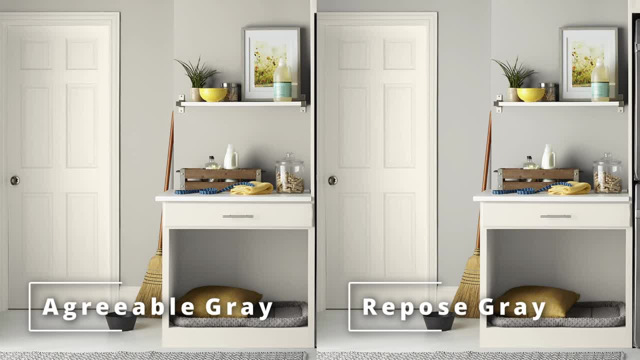 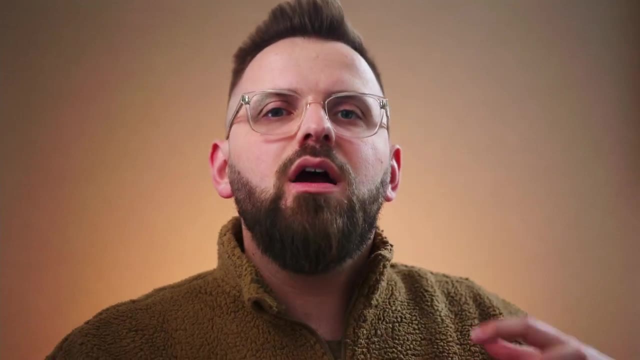 which makes them lighter, mid-tone colors. This also speaks to their popularity, because colors around that 60 light reflectance value tend to be used more often than dark colors, especially on things like walls on the inside of your home. This is because they tend to feel a little more. 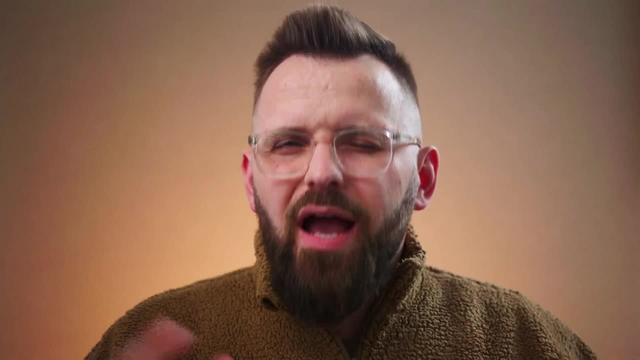 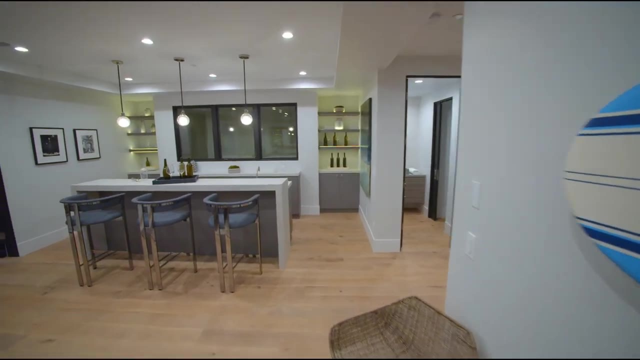 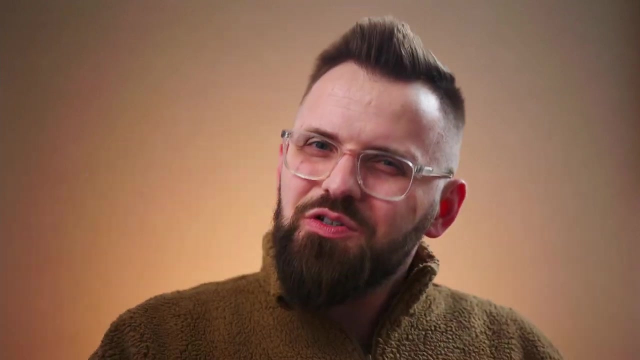 light and airy than some of their darker counterparts. There has been a bit of a resurgence of lighter colors becoming more popular, especially for those people that like a more understated minimalist look. But the only issue with going with a lighter color, especially one that's like 80 plus LRV, is its undertones. 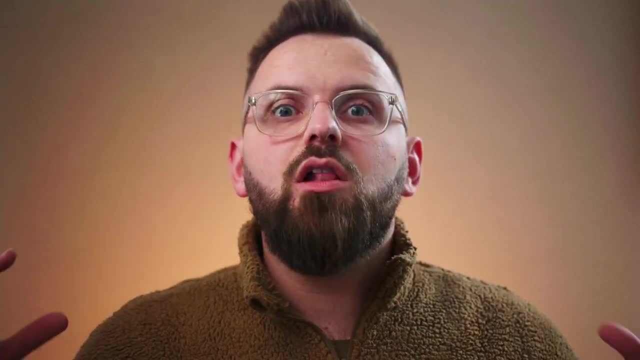 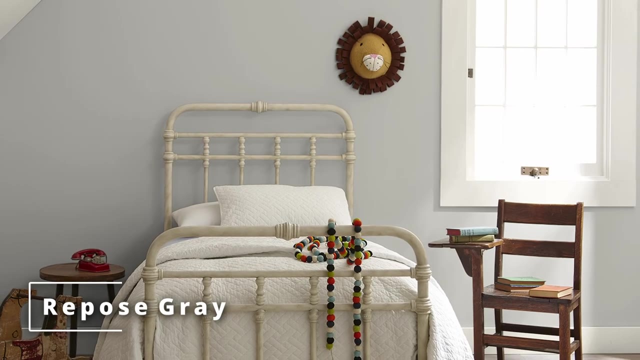 won't be as visually apparent, especially if there's a lot of light surrounding it to wash the color out. Colors like repose gray and agreeable gray sit in that little sweet spot, that sort of Goldilocks spot where it's not too dark or not too light in most cases. I would even 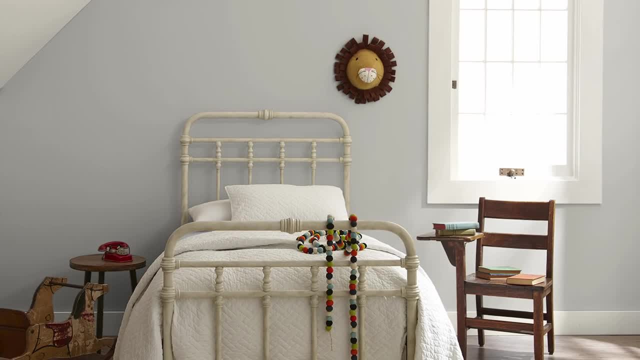 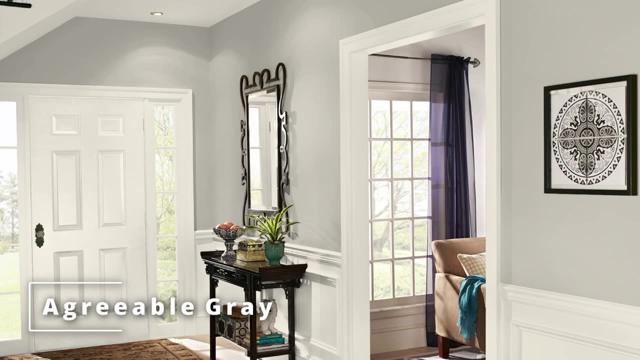 use these colors in identical situations. They're great in bedrooms. you can use them in bathrooms. they're even suitable for the main arteries of your home, like your hallways or those more open living and dining rooms. You could really make a case for them to be a little bit more. 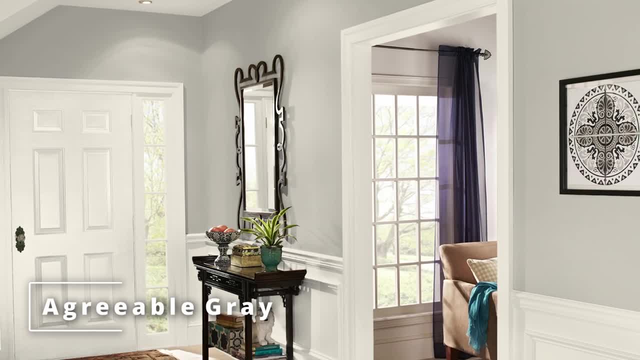 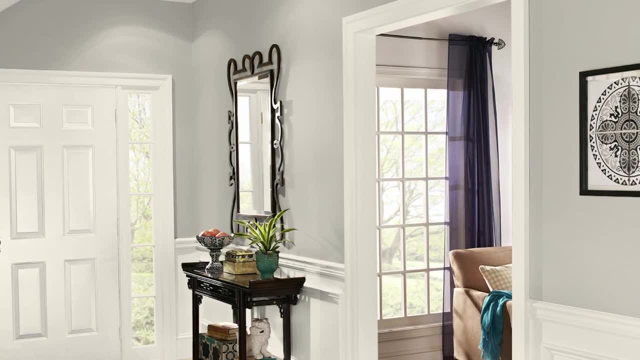 colorful. You could make a case for any room in your home for either of these colors and no one would bat an eye. Some of the reasons I could see people not using these colors in certain rooms is if they maybe wanted to- I don't know- change things up and pick something a little more dynamic or saturated. 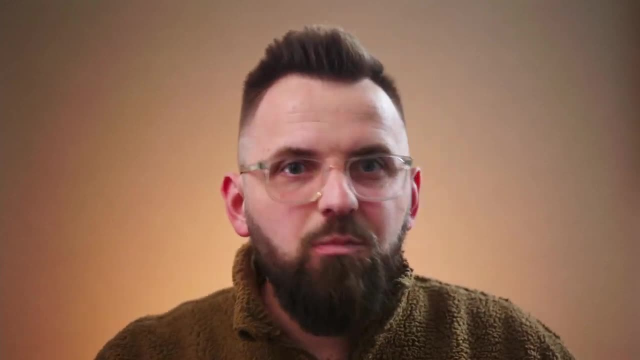 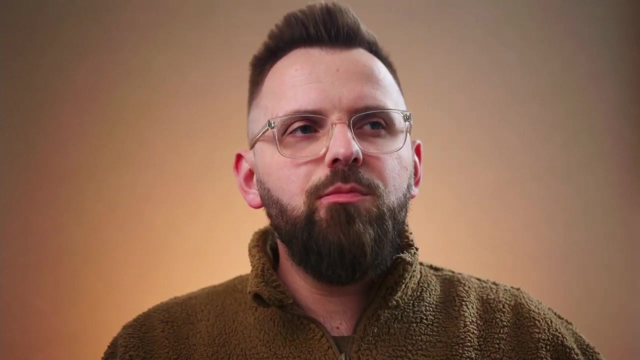 like some brighter colors or deeper based taupes or navies or forest greens, Anything that you might deem as an accent. There are also certain situations where you have a room that maybe gets little to no light and could perhaps be a little bit too dark or too bright for your home, If you're looking for a room that's a little bit brighter or a little bit darker than your home. you might benefit with a color around a 70 or even an 80 LRV, just to keep things feeling as light as possible. Now, even though these two colors are super similar, they both exist for a reason. They're not totally 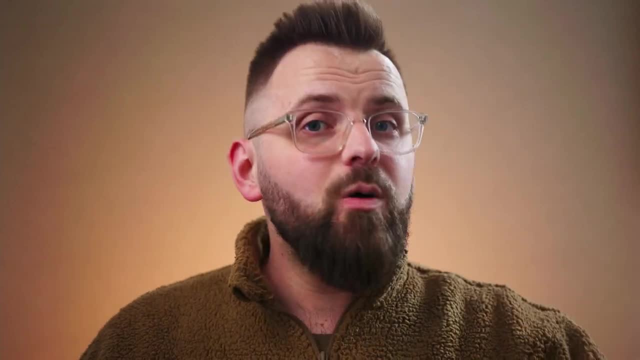 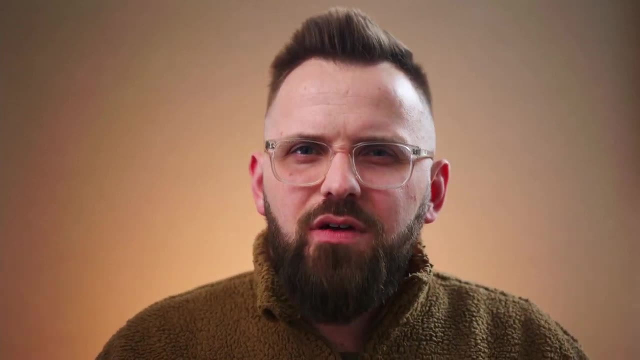 redundant. They're not identical and one could very well be better than the other for whatever project you're doing. So even though they're both classified as gray, you could argue that they fit into the grayish category, which is a combination of gray and beige, Repose and Agreeable Gray. they both offer slightly different colors, but they're both very similar in color. They both offer slightly different colors, but they're both very similar in color. You could argue that they fit into the grayish category, which is a combination of gray and beige, Repose and Agreeable Gray. they both offer slightly. 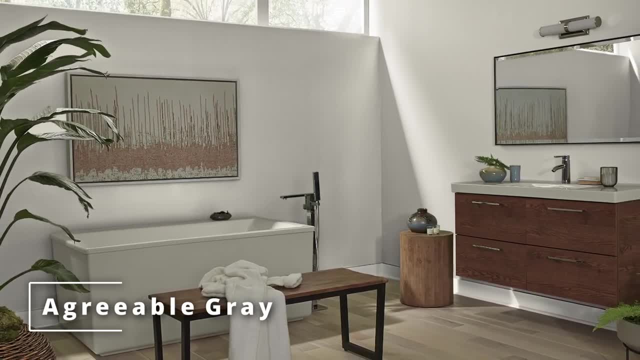 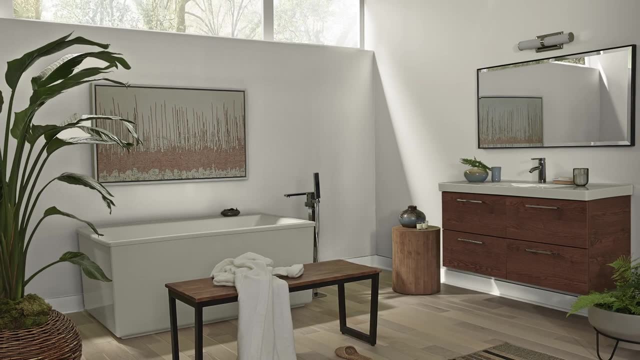 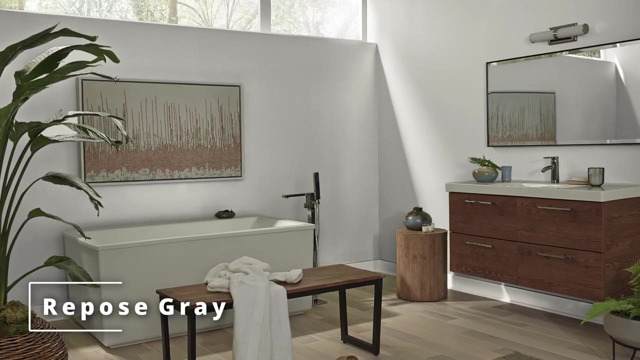 different ratios of one and the other, To me Agreeable. Gray almost appears a touch closer to taupe, which is a combination of gray and brown, while Repose Gray is a little more gray, with just a touch of beige, almost giving it a hint of a green undertone in certain cases. Objectively, 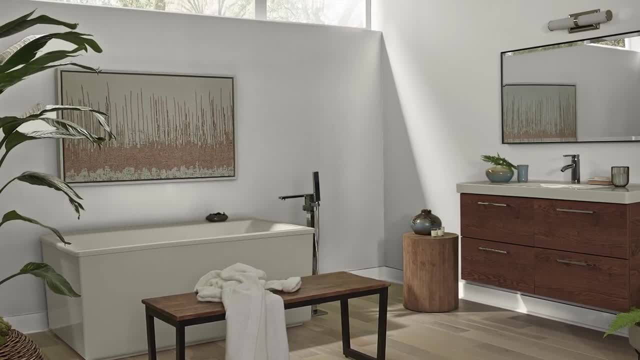 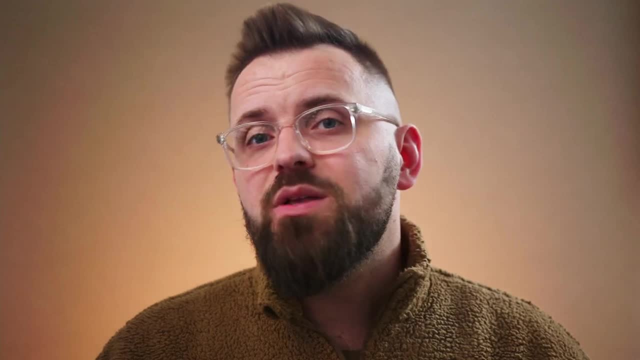 on their own in a neutral environment. they do tend to have a gray aesthetic, but just keep in mind that both can have a tendency to show a tiny bit of green, depending on the color, For example, if you have a lot of reds or purples, or like a beautiful natural brick. 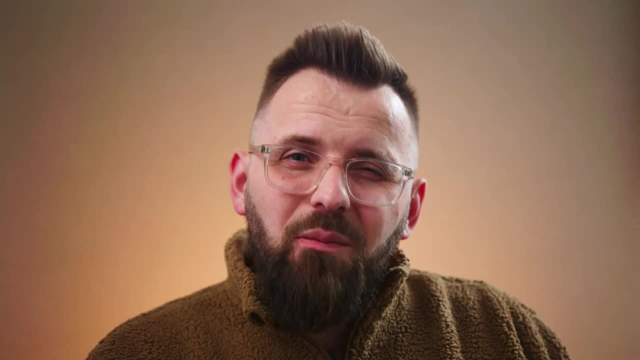 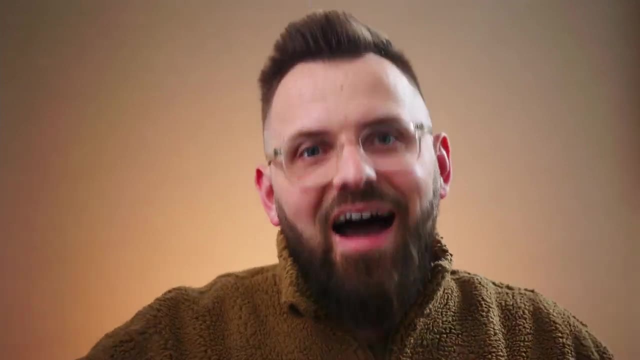 wall or something on the inside, you might see some of that green pop up a bit more in almost a complimentary fashion. Or if you're a fan of really cool bluish lighting with a high kelvin value, similar to daylight, that could also have an impact. 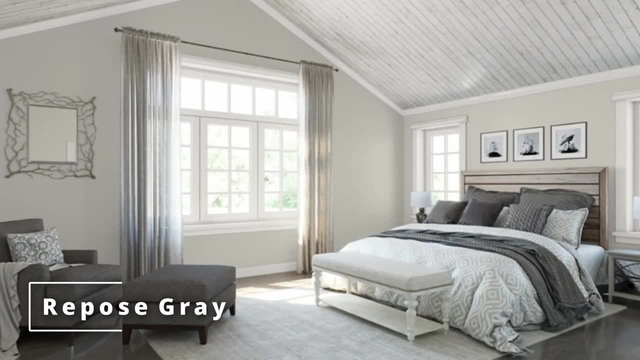 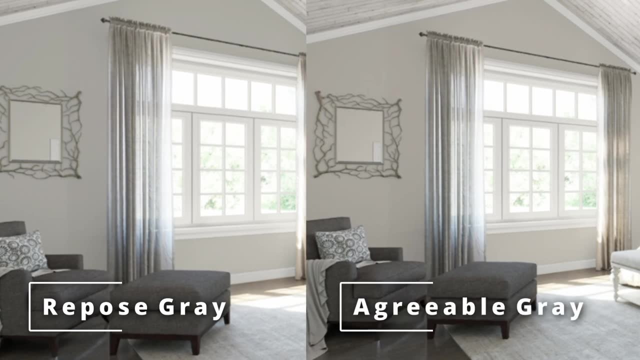 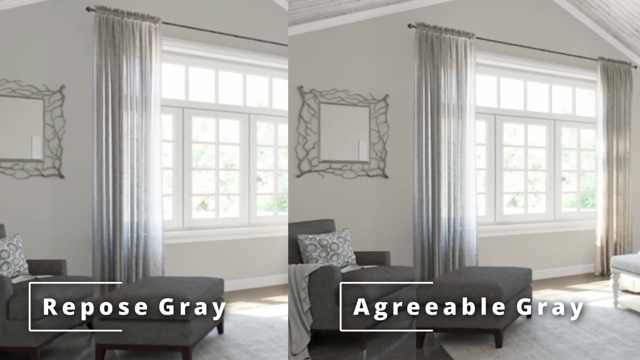 So the first big difference is: Repose Gray is just a bit more gray, or at least in the traditional cool gray sense. It has a bit less of that red brown undertone found in Agreeable Gray, and that's enough to split the difference. Back on the subject of light reflectance value, or 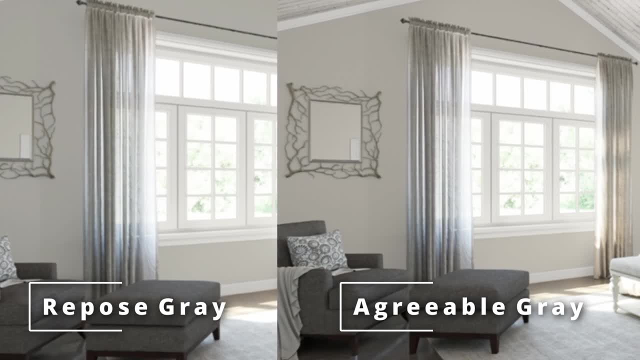 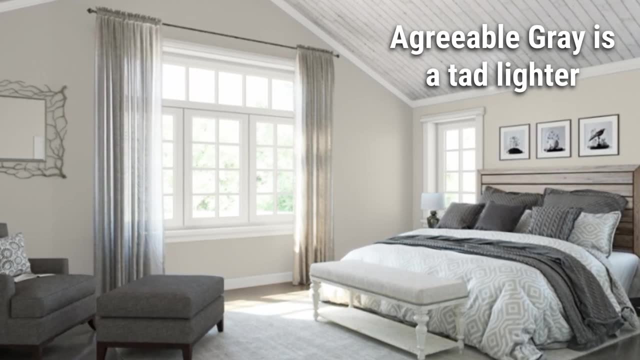 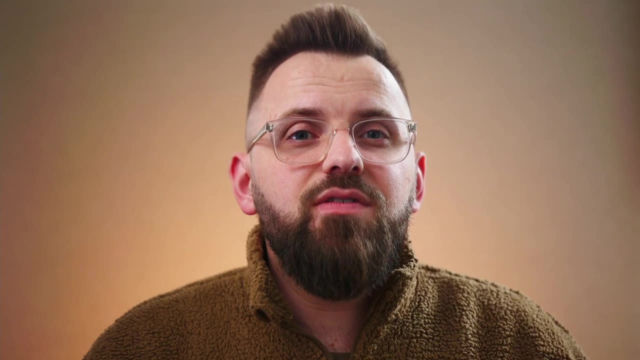 how dark each color is compared to one another. they're extremely similar but technically not identical. Agreeable Gray is just a tad lighter with a 60 LRV compared to Repose Gray's 58 LRV. So if you love both colors but just wanted something to feel a tiny bit more, 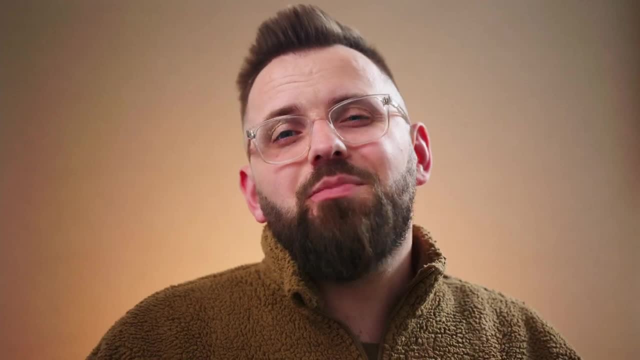 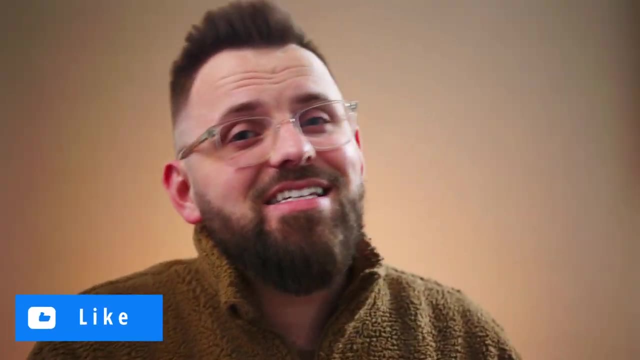 airy and open, then that would be Agreeable Gray, but it's a close one. It's only a two point difference. What about my opinion on these two colors? Well, I think in certain cases, each one can really be a phenomenal choice for both inside and outside your home. I do find 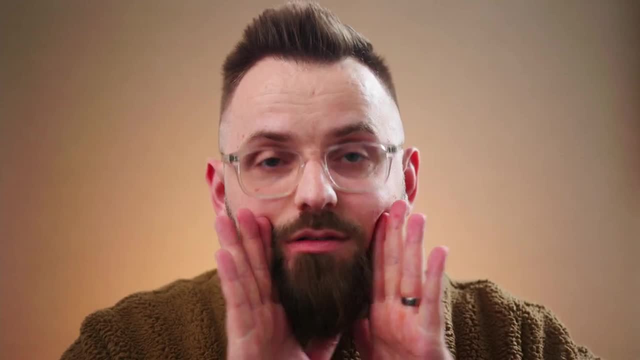 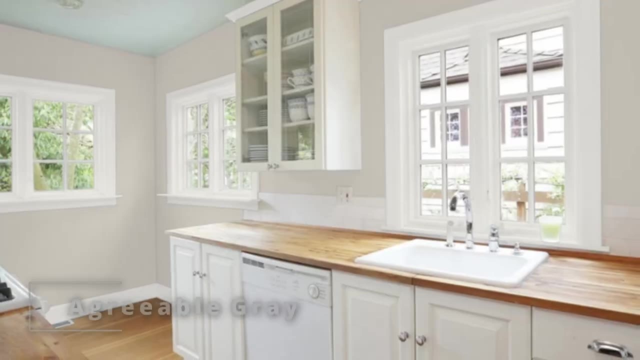 Agreeable Gray to just be a bit more agreeable There. I said it Especially if you do incorporate more brown tones in the form of wood, for example. If you have a lot of wood, the brownness in Agreeable Gray will just work out better. But if you have a lot of wood then you'll have to go with. 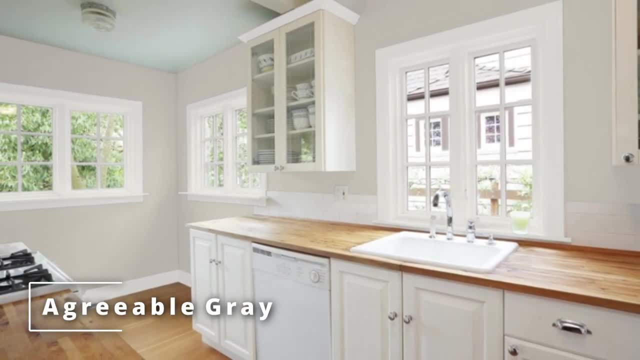 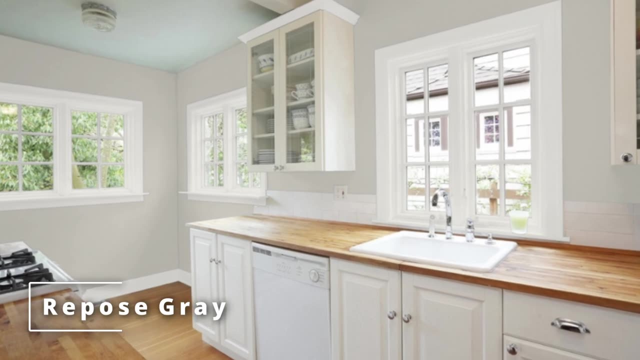 a little bit easier, while repose gray will just sort of complement a little bit more. You could also say that repose gray would maybe seem to fit seamlessly with the cooler color schemes or people that are fans of green or metallics, but really it just depends on your. 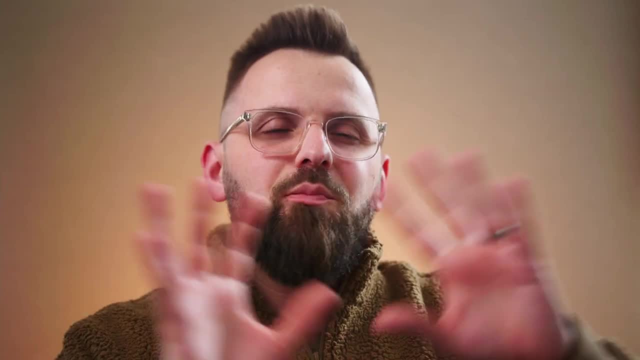 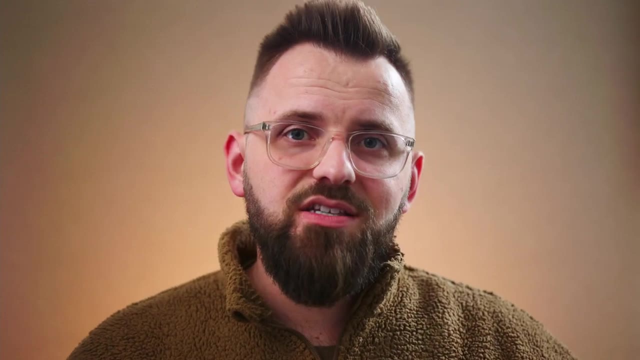 overall design plan. Maybe you do want a little bit of a back and forth, or you want something that's a little more adjacent, or even monochromatic in your color scheme, I think. in most cases, though, if you're torn between the two, it really is kind of a 1A, 1B type of scenario. 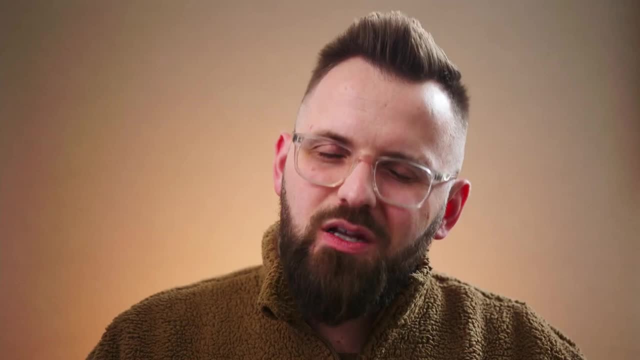 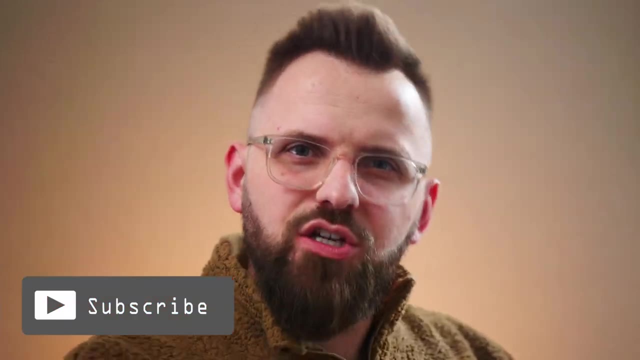 Testing them out is going to give you the confidence you need to really solidify your choice one way or another. So it's just a step that you sometimes can't skip. Another way testing helps you out is by showing how much light actually affects colors, including these two. And we talked about that in a video right over here.